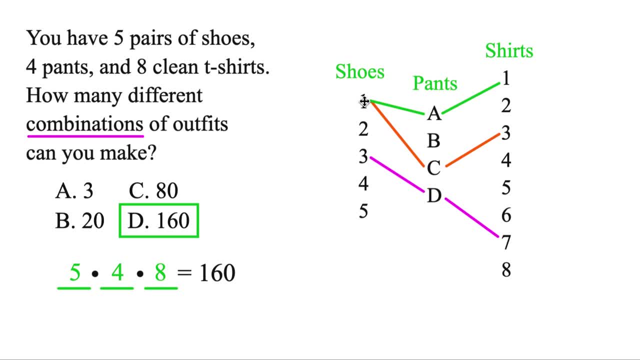 Now you could visualize this, because when you go from the left side to the middle, to the right side, that's one specific combination, but every time you go from the left to the right, that's another one, and there's going to be a lot of them. 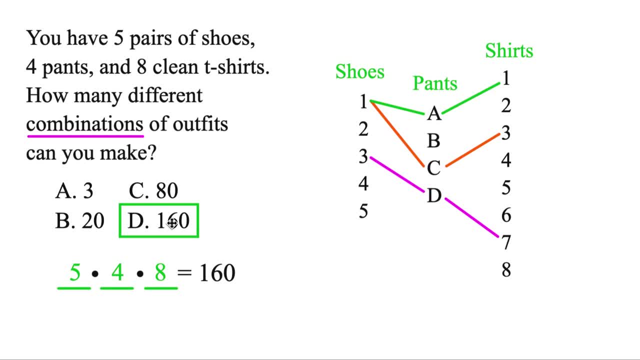 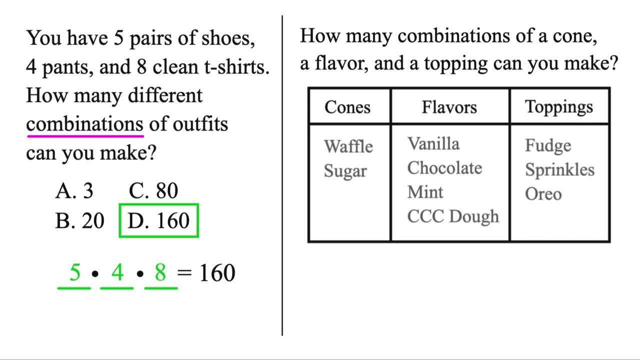 So therefore there's exactly 160.. Okay, feel free if you want to pause and practice with this one. We know it's a combination, It's going to be multiplication. so two times four times three, just like that, and if you got 24,, bingo. 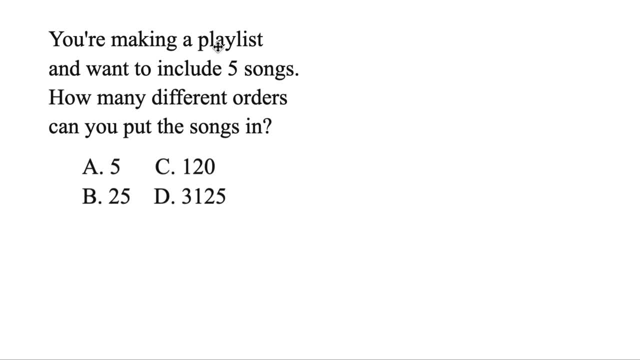 Another type of question you could get. you're making a playlist. You want to include five songs. How many different orders can you put the songs in? The keyword is order, so we'll put five spots for the five songs. How many ways could we choose that first song? You could choose any of the five. 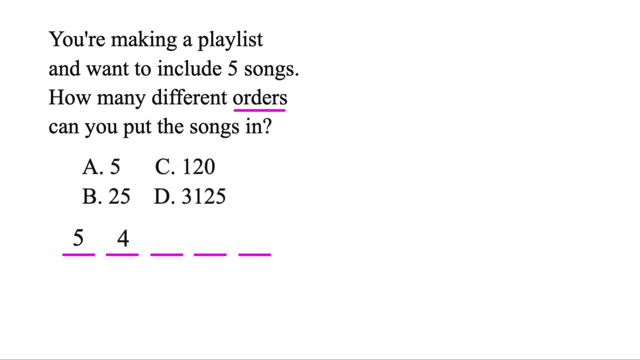 but once you choose that one, then you've only got four remaining from there. you choose your second song, you've only got three remaining from there, and so on, all the way down to one. Once again, we're going to multiply these together, so that's going to give us 120.. 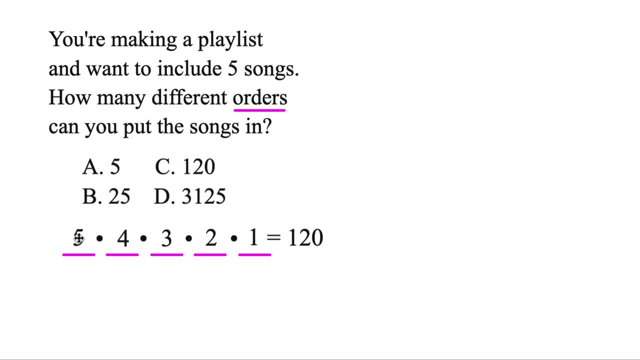 So if you're finding out how many orders of things, you just start with that number, multiply down to one and boom, You got it. Now you could again see how many there really are by writing out incident. So if you're gonna multiply all of that together, you want to. 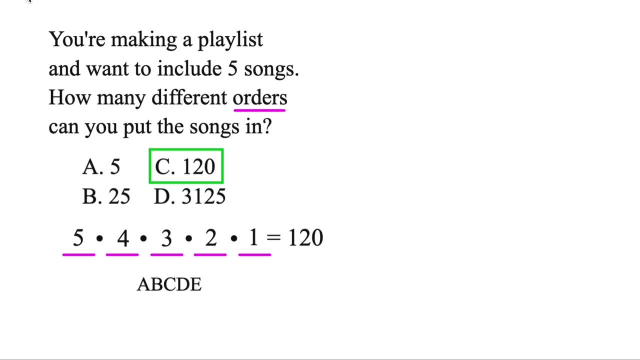 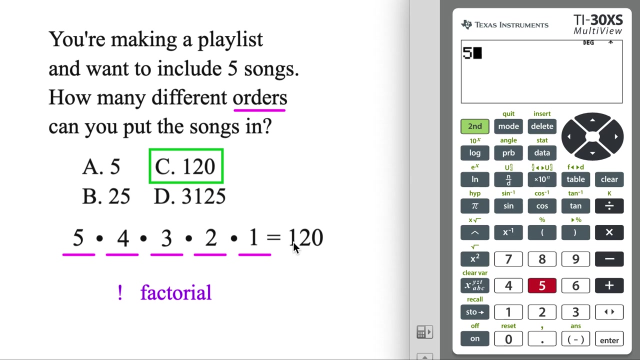 out ABCD as the five songs, but you switch any of them, then that's a new order, that's a new playlist. keep going, there's gonna be 120 total. another way to use the calculator for this is there's a shortcut. we could use the factorial button. so, for instance, if you don't want to multiply 5 times 4, all the 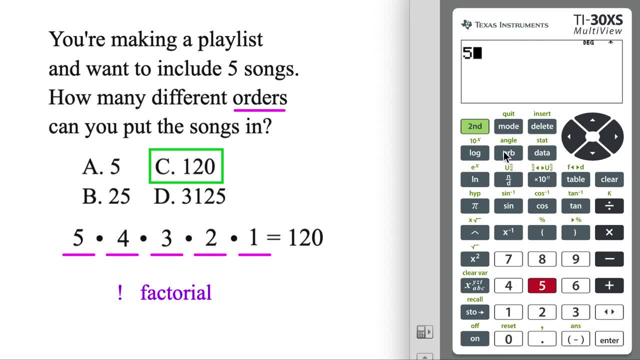 way down. you could just do this exclamation point. it's in the PRB or PBR button there for probability, and then you go down to the exclamation point. and, by the way, the way that you say that is, it's just 5, but you have to. 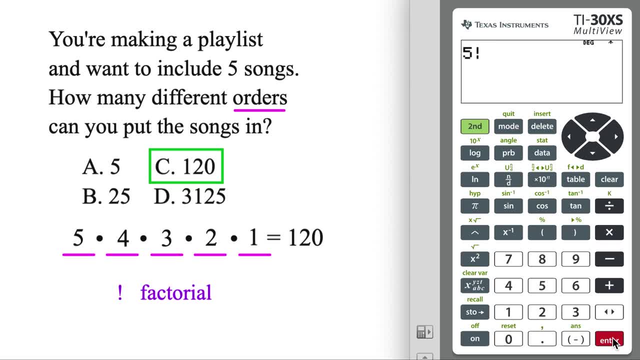 yell it. that was a joke. okay, that'll give us 120, and that's the exact same thing as what we did over here. we just didn't have to type in the whole thing. it knew what we were doing. so that's the exact same thing as what we did over here. we just didn't have to type in the whole thing. it knew what we were doing. so 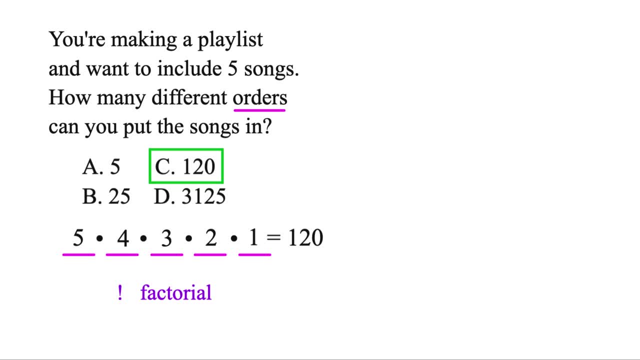 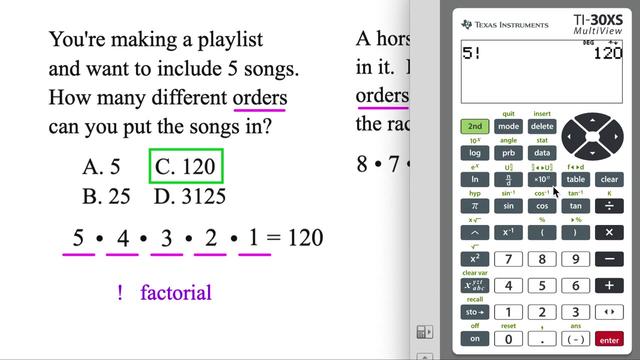 that's another way to get 120. okay, feel free to pause if you want to practice with this one. here you got it. you know it's order. you know there's eight things. you're just gonna do eight times seven all the way down to one. but you might have thought I think I. 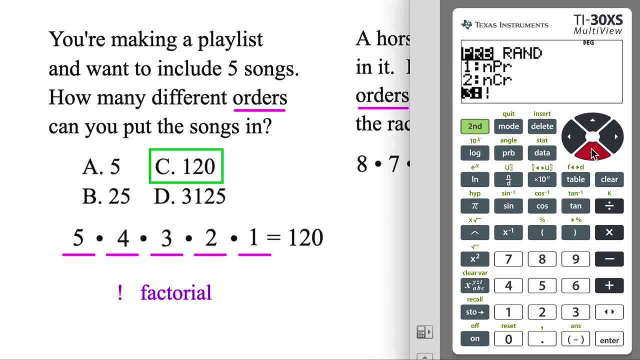 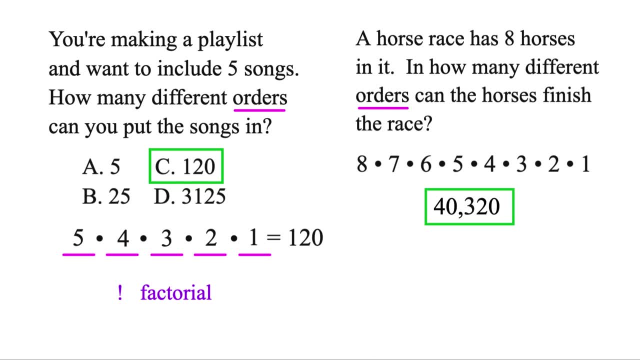 messed something up, my numbers too big. now you did it right, it's just pretty. extra forty thousand three hundred twenty, that's how many orders these horses could finish. extra forty thousand three hundred twenty, that's how many orders these horses could finish. now what if you're interested in just the first, second and third place, then 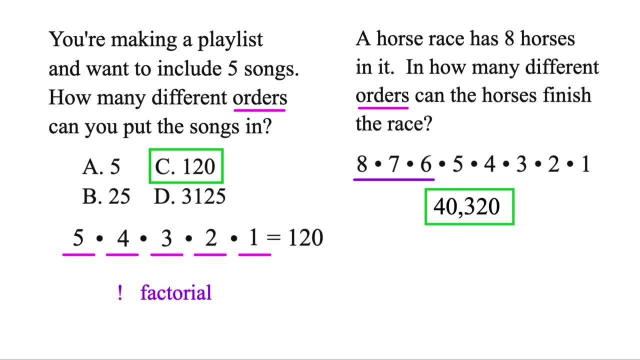 you're just going to multiply the first three numbers, so in this case that would get us three hundred thirty six ways for them to finish in the top three. if you're at a horse track and you're making a bet, this is called a trifecta bet, even if 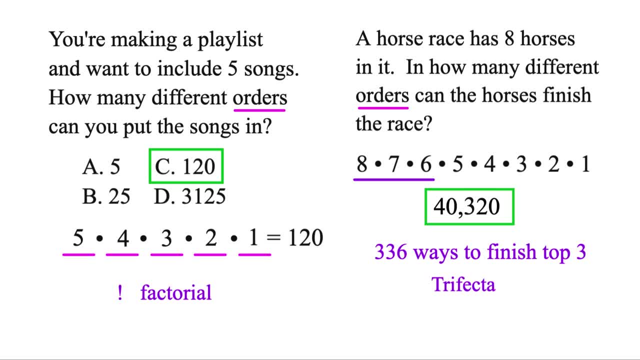 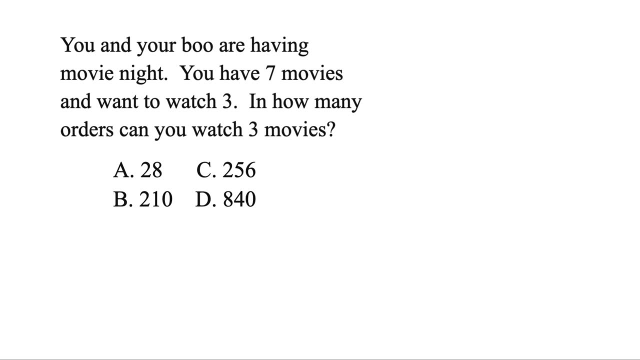 you put down a one or two dollar bet, but you got it right. the payout would be probably a couple hundred, maybe even thousands of bucks. extremely unlikely, so good luck. you and your boo are having a movie night. yeah, have seven movies. you want to watch three. how many different orders can you watch three movies? well, let's pretend we're. 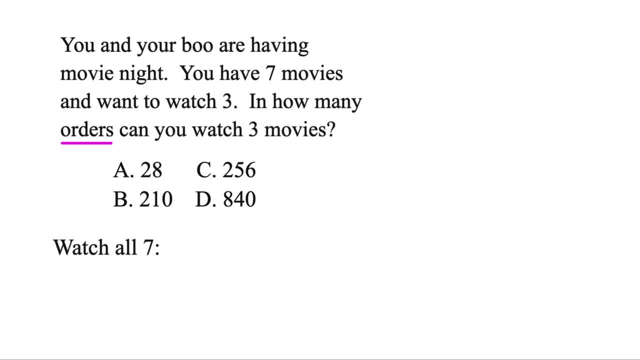 watching all seven. we know it's the order of them matters, so we'll multiply them down from seven down to one. but just like the horse race, If we're only interested in the first three, then we're just going to multiply seven times six times five. 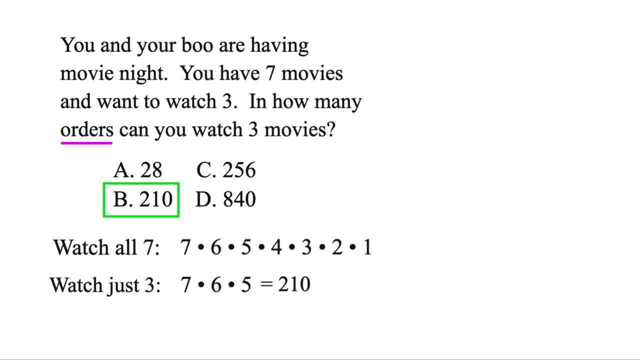 In that case, it'll give us 210, and that's it. So how many ways can we watch three movies if you're given seven? That's it. And you can only watch 12 hours straight of Lord of the Rings Extended Edition, so that's. 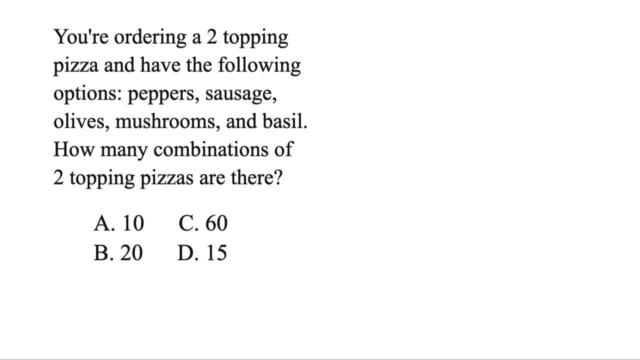 why we're not watching four, Three's enough. You're ordering a two-topping pizza. You have the following options: peppers, sausage, olives, mushrooms, basil. How many combinations of a two-topping pizza are there? Well, you could do this one by hand, because you could say: peppers, sausage, peppers, olives. 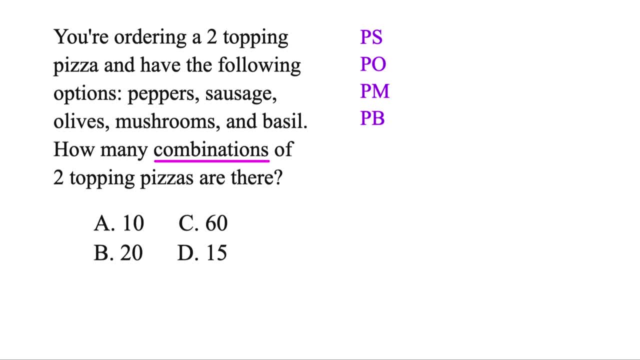 and just keep going from there. All the pepper combos are these ones. Then, when you pick up with sausage, you don't want to go backwards because you already have a pepper-sausage combo there, So you just move forward. Sausage-olives. 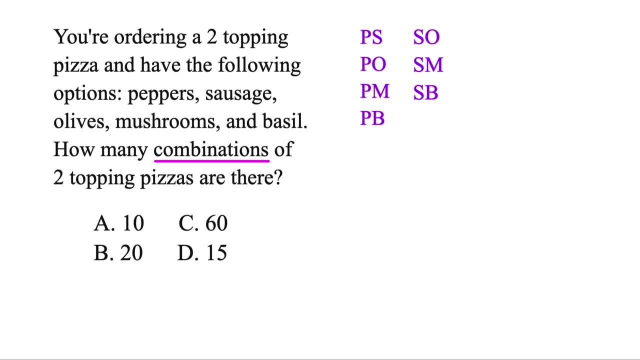 And so on. So those are all the sausage combos And the olive combos. there'll be two more of those. And finally, mushroom-basil Sounds pretty gnarly and that's our last one. Counting these up, there's going to be ten of those. 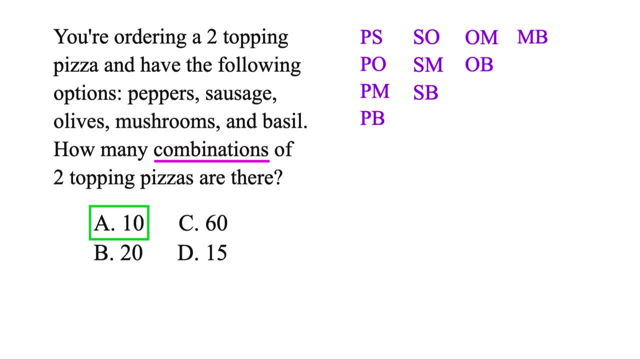 So therefore, ten combinations are possible, But that can be kind of a pain, so lucky for us, there's a way to do it with the calculator. When you're choosing a small group from a larger group, You could use this NCR button. 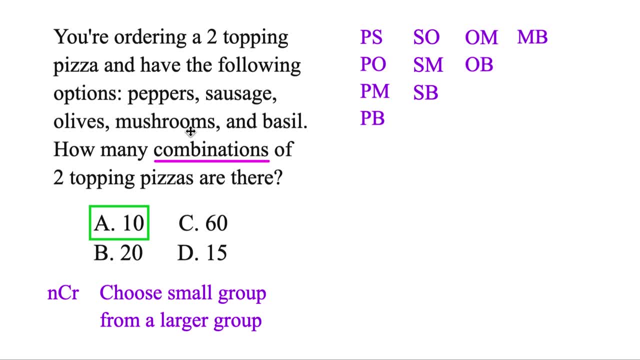 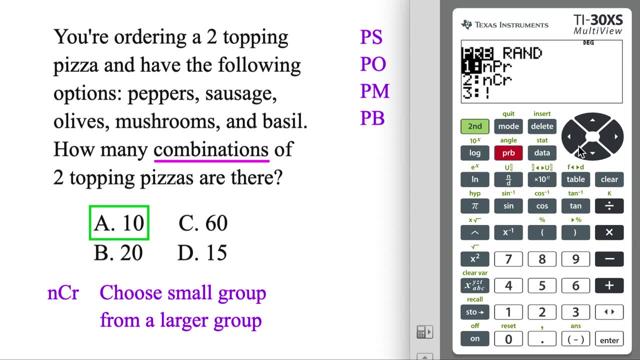 In our case, we have five things. that's the large group, But we're making a smaller group of two from that. So therefore, you'll start with the bigger amount, the PBR, button down to NCR. How many groups of two can we make? 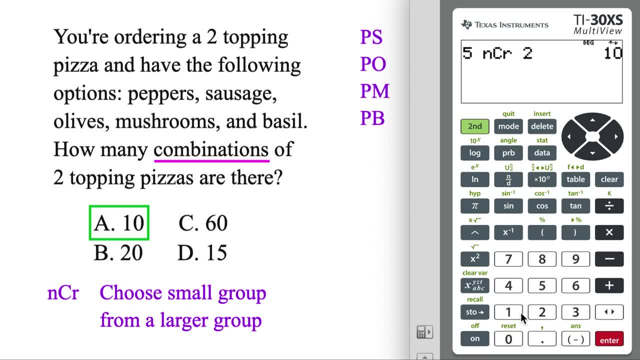 That's another way to get ten, just like that. So for instance, let's say, ten people are auditioning as extras for a movie, but there's only four spots available. So how many ways can we form a group of four out of ten? 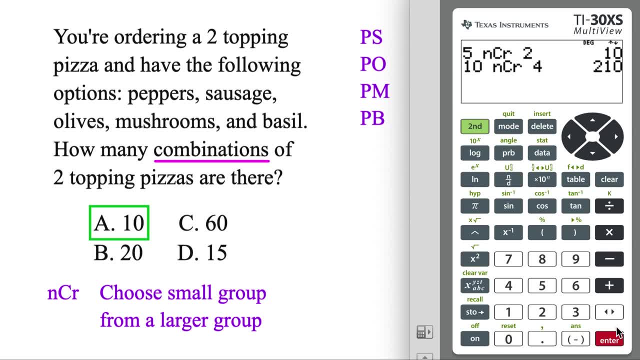 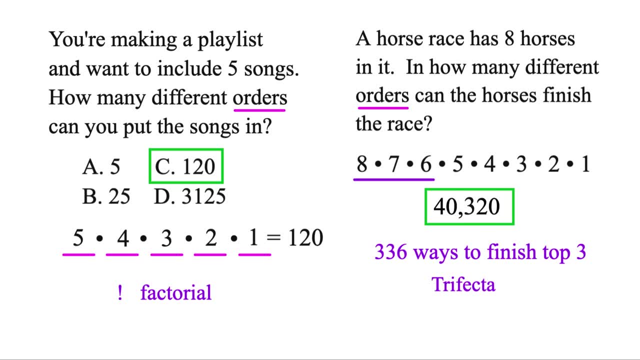 There'd be 210 different ways to get a group of four Between these. these are the main types of combo and order problems that show up on the GED. You got these Good luck. We'll see you in the next video. Toodles.